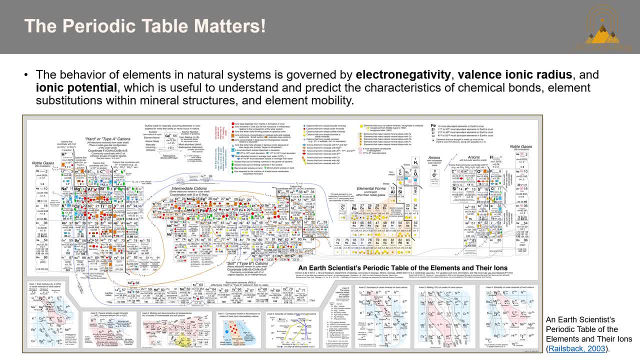 I chose to use this image over a standard periodic table because it presents the naturally occurring charge species commonly encountered by geoscientists, as well as elemental forms, and it's organized by charge. Organized by charge yields an arrangement more conducive to recognizing geochemical trends and provides a framework for understanding the geochemistry. 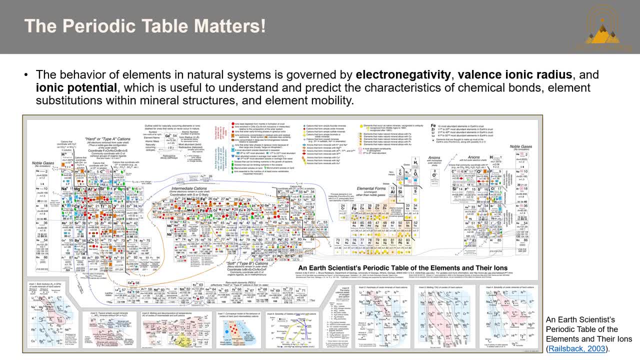 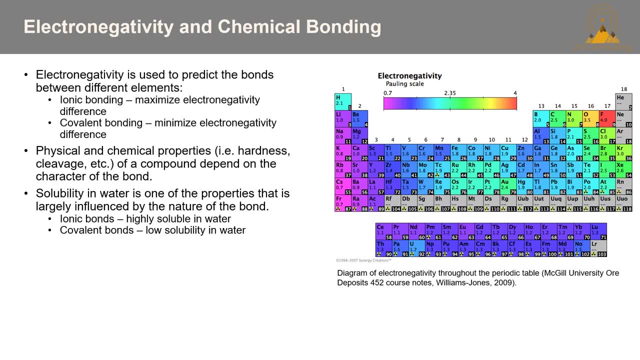 better than the conventional table. The first topic I'm going to touch on is electronegativity, a word that you'll likely know but may not recall why it's important in the context of geochemistry. It's a useful concept for the following reasons: It's used to predict bonds between different elements. 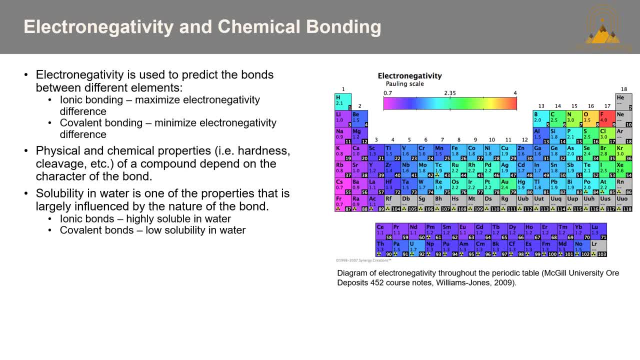 whereby ionic bonding has high electronegativity difference and covalent bonding minimizes the electronegativity difference. Physical and chemical properties, including hardness and cleavage, become powerful in the case of geochemical trends- The first topic I'm 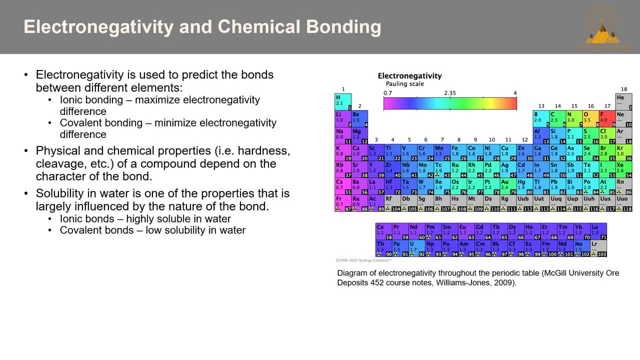 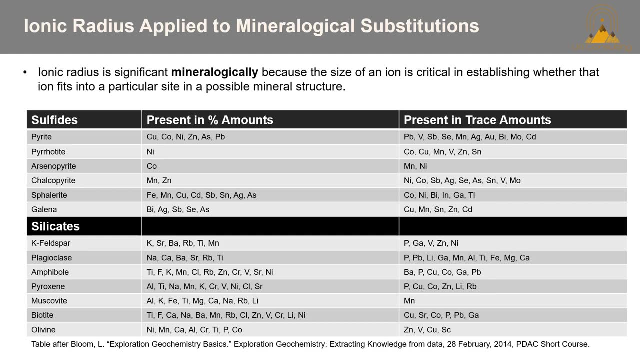 going to touch on is ionic bonds. Ionic bonds depend on electronegativity and the solubility in water is largely influenced by the nature of the bond, whereby ionic bonds are highly soluble in water and covalent bonds have low solubility in water, Following this ionic 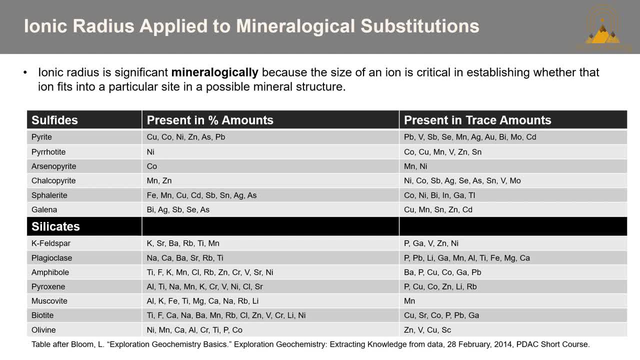 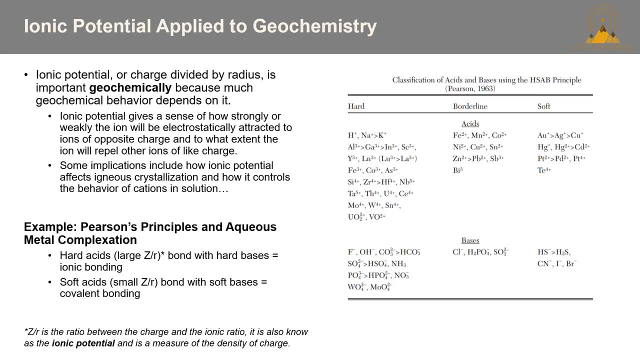 radius is important mineralogically because the size of an ion is critical in establishing whether that ion fits into a particular site in a possible mineral structure. The table below is a great summary of the two Ionic potential or charge divided by. radius is important geochemically because much of 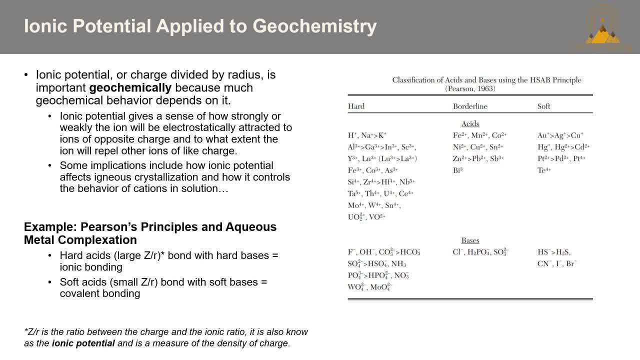 the geochemical behavior depends on it. Ionic potential gives a sense of how strongly or weakly the ion will be electrostatically attracted to ions of opposite charge and to what extent the ion will repel other ions of like charge. Some implications include how ionic potential 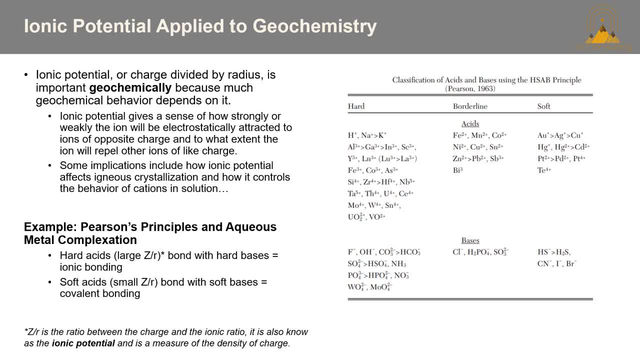 affects igneous crystallization and how it controls the behavior of cations in solution. A great example of ionic potential in practice are Pearson's principles for hard- soft acids and bases, which is applied to metal complexation. There are an appreciable number of ligands. 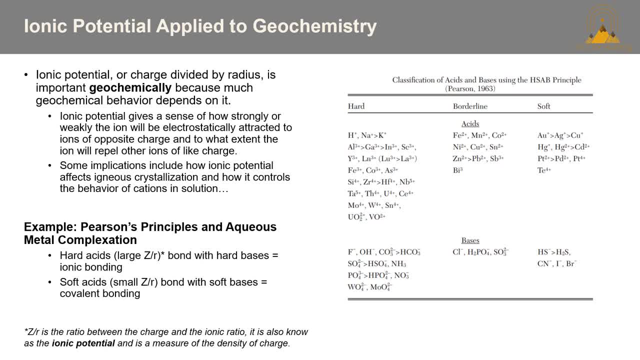 that can facilitate metal transport by hydrothermal fluids by forming metal complexes. but the important question for economic geologists are which of these ligands form stable complexes within the metals of interest. Ionic potential is important geochemically because ionic bonds are highly soluble in. 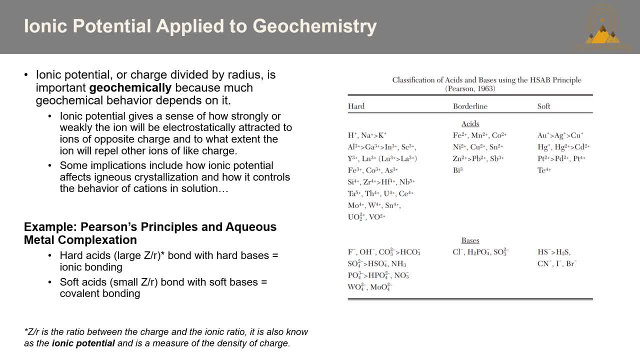 gas and can play a role in their transport. Pearson proposed that, in the case of competition among ions, hard acids or metals will bond preferentially with hard bases and do so ionically, whereas soft acids will bond preferentially with soft bases and do so covalently. 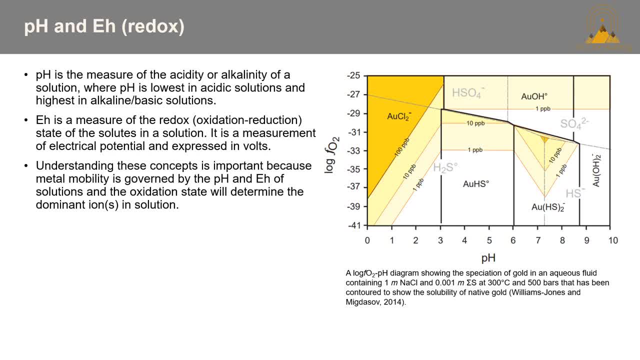 Knowledge of redox conditions or, equivalently, oxygen fugacity and pH at which rock forms and evolves, is important for interpreting the rock's history. pH is a measure of the acidity or alkalinity of a solution, where pH is lowest in acidic solutions and highest in alkaline or basic solutions. 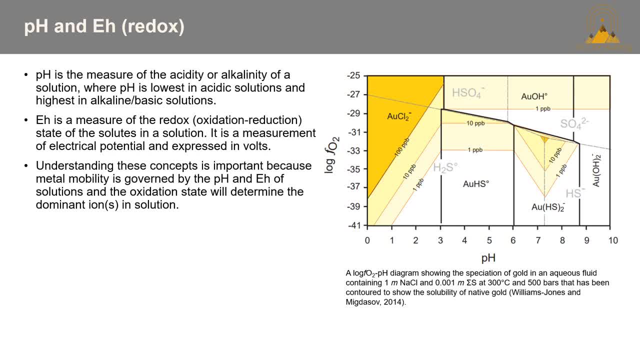 EH is a measure of the redox or oxidation reduction state of the solutes in a solution. It is a measurement of electric potential and is expressed in volts. Understanding these concepts is important because metal mobility is governed by the pH and EH of solutions and the oxidation state will determine the dominant ion or ions in solution. 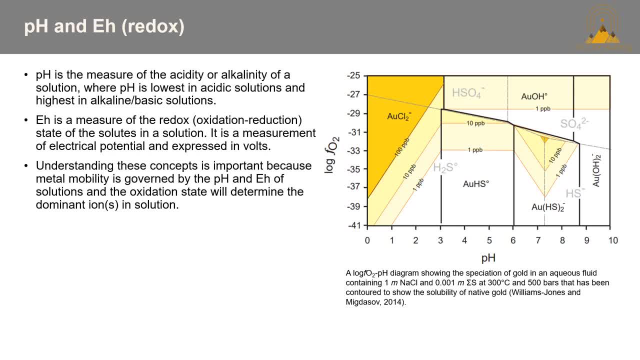 The diagram at the right shows a system at 300°C and 500 bar. It illustrates fields of stability where gold can be transported as specific complexes, For example AuCl2 at a pH of less than 3 over a range of oxidation states, whereas AuHS2- between a pH of approximately. 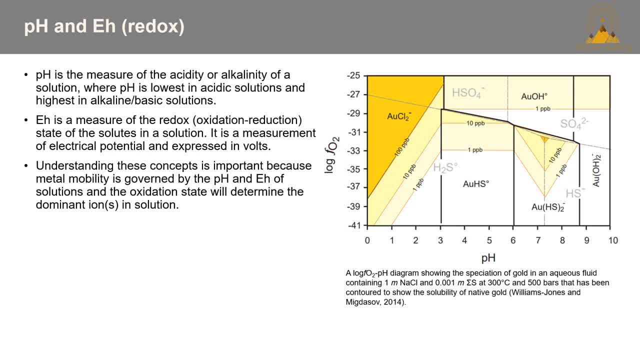 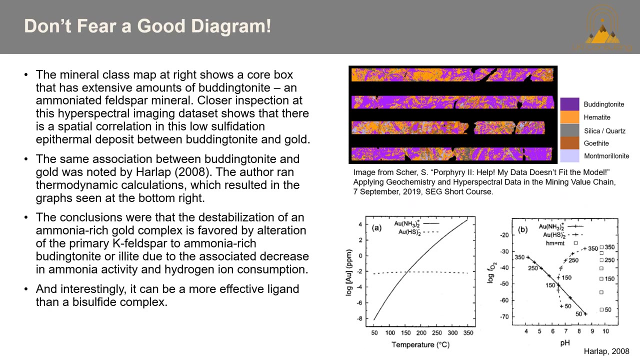 6 to 8.5 in more reducing conditions, And superimposed on this diagram are contours for solubility of gold and the conditions that need to be met for it to precipitate from solution, and in what quantities. In the last slide we talked a bit about LOGO-FO2 pH diagrams and it wasn't too scary, hopefully. 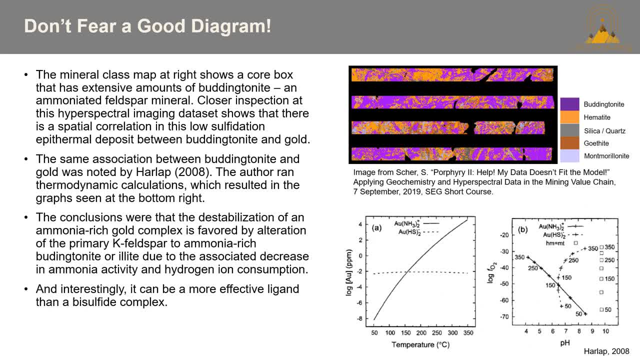 helpful. Here we'll have a look at a real-world geochemical mineralogical data with some theoretical diagrams built on simple thermodynamic calculations. The mineral plasma up at right shows a core box that has extensive amounts of buddingtonite. You can see this in purple. Buddingtonite is an ammoniated feldspar. 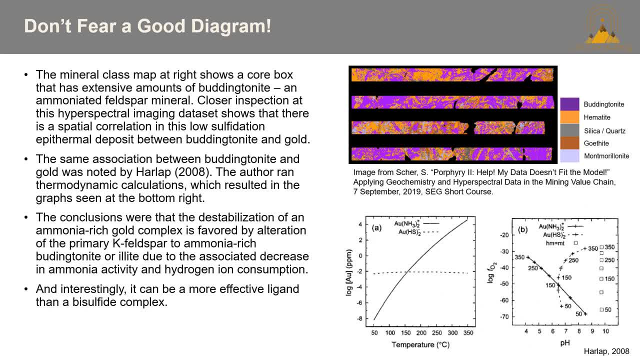 mineral. At closer inspection in this hyperspectral imaging data set we can see there is a spatial correlation in this low-sulfonation epithermal deposit between buddingtonite and gold. The same association between buddingtonite and gold was seen in the first slide. The same 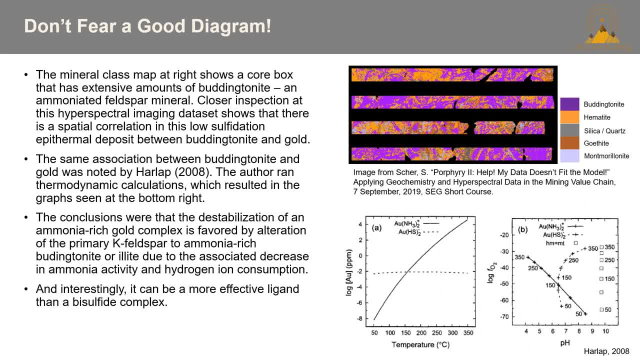 association between buddingtonite and gold was seen in the second slide. The same association between return on phase and neg quotidies was noted by Haslott 2008.. The author ran thermodynamic calculations, which resulted in the graph seen at the bottom right. 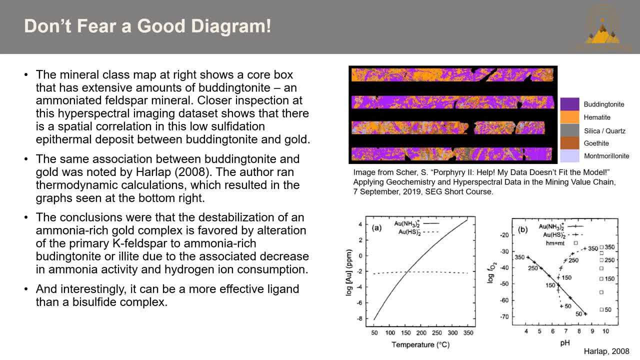 The conclusions were that the destabilisation of an ammonia-rich gold complex is favoured by alteration of primary K-feldspar to ammonia rich buddingtonite or illite, due to the associated decrease in ammonia activity and hydrogen ion conception Inspired by a gas, both ionic and sodium gas constituents겁ic acid. 엄청 Hotel, we just saw attention. 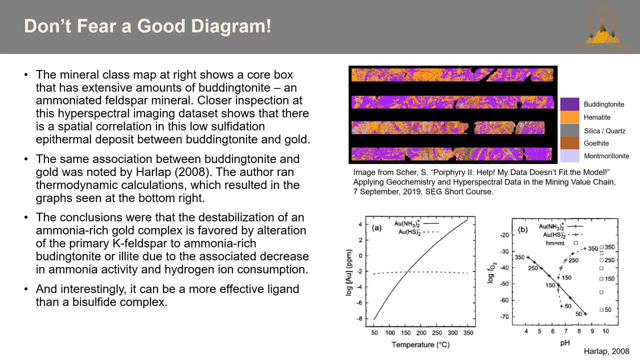 to this above here in the graph, but at least we can see a sticky spring� And interestingly it can be a more effective ligand than a bolactin. Cab examines there, judging a ELSA chemical property to structuresuciones. 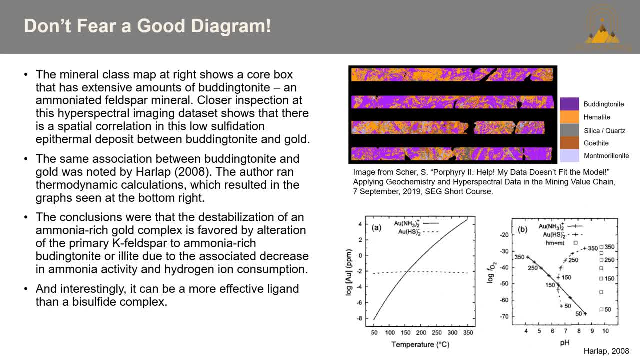 JO1DI133.. JO1DI133.. JO1DI133.. JO1DI133.. JO1DI133.. bisulfite complex. So, as you can see in the diagram to the right, we have log AU PPM versus temperature And, at temperatures at about 150 or greater, the ability for the ammonia ion to 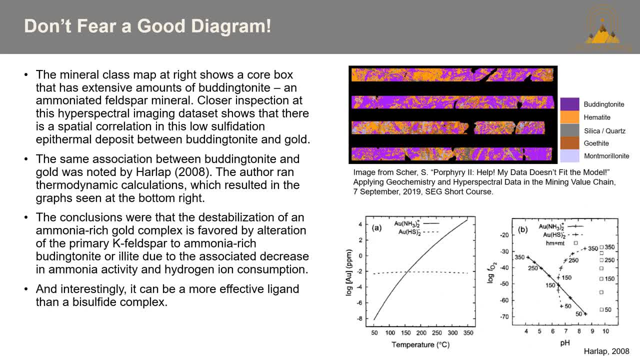 transfer gold is significantly greater than it is for the bisulfide. Looking further to the right, we have a log FO2 versus pH diagram where you can see that at pHs less than about six and a half and more, slightly reducing to more oxidizing conditions that the ammonia ion is also. 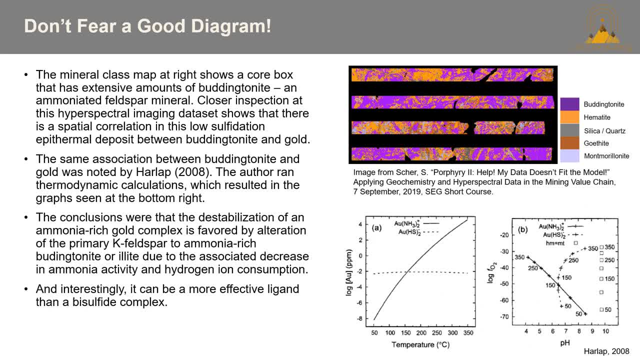 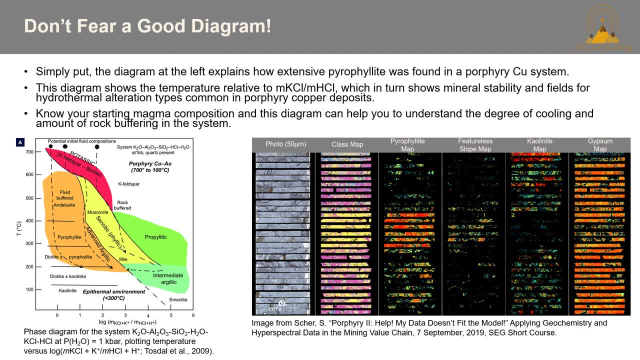 great at is better at transporting gold. Simply put, the diagram at left explains how extensive porphyry was found in a porphyry copper system. The diagram at the left shows the temperature relative to MKCL over MHCL, which in turn shows: 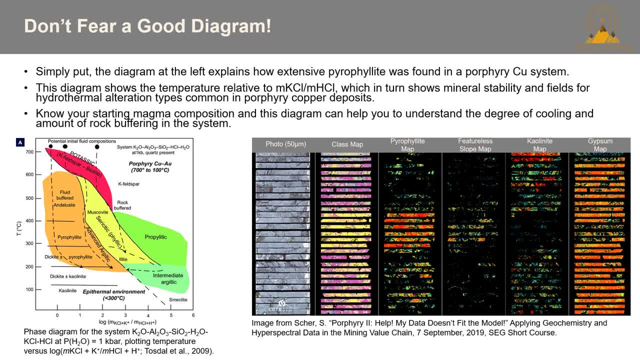 mineral stability and fields for hydrothermal alteration types common in porphyry copper deposits. If you know your magma, your starting magma composition, and this diagram can help you understand the degree of cooling and amount of rock buffering in your system, For instance. 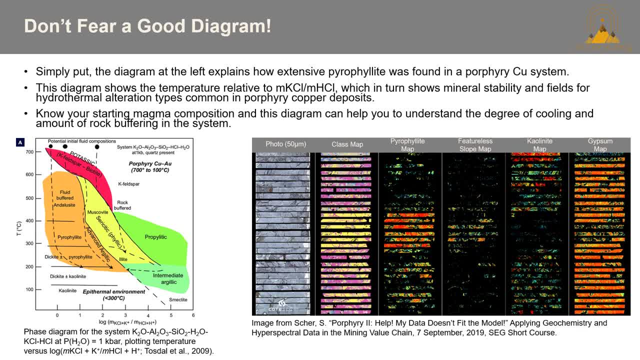 in the image at the right, you can see rocks with a large amount of prophylate in them. these rocks are also from about a kilometer depth. Referring back to the diagram at the left, you can observe that, starting with a magma composition that has a lower K over NA composition, 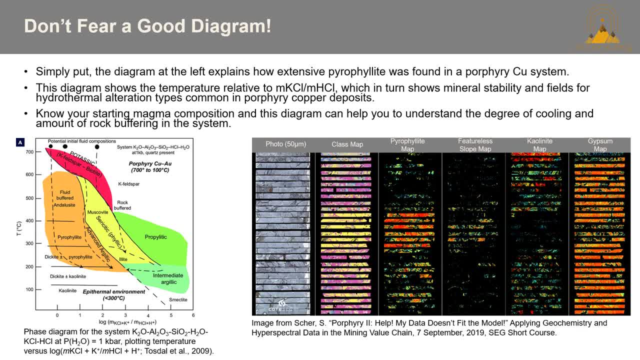 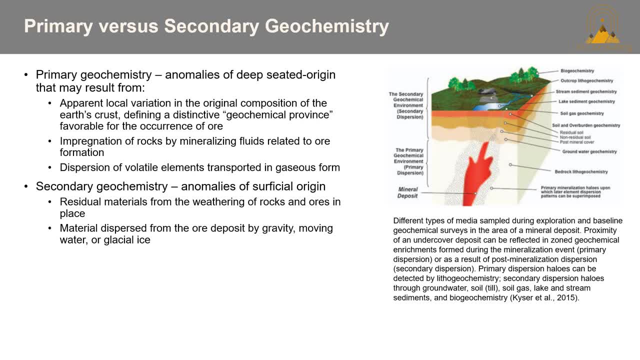 as you cool it, you pass through the stability field of prophylate Switching gears. it's important to talk about what you're going to be tracking in your geochemical data set, Namely our geochemical data set. The geochemical data set is the geochemical data set that is used to 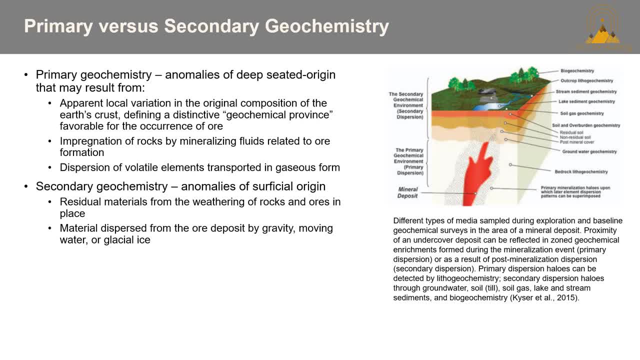 determine whether you're looking at primary or secondary geochemistry. For primary geochemistry, we're looking at anomalies of deep-seated origin that may result from apparent local variation in the original composition of the earth's crust, defining distinctive geochemical province favorable for the occurrence of ore impregnation of rocks by 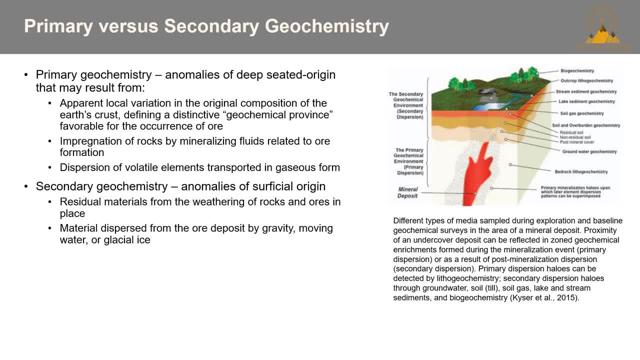 mineralizing fluids related to ore formation, or also dispersion of volatile elements transported in gaseous form. For secondary geochemistry, these are anomalies of circular formation, slanged as prisingly boat train� wrote in court. As such, the geochemical data sets will take place within trimming of theorer origin. 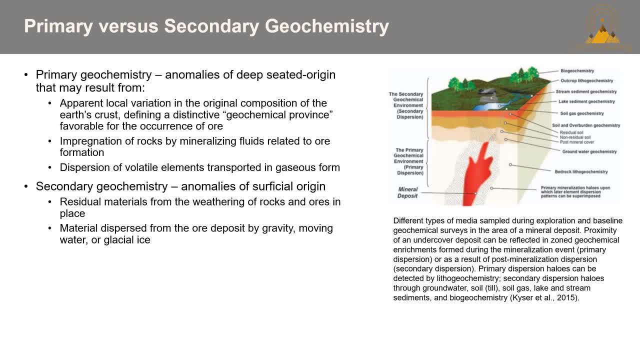 Residual material from the weathering of rocks and auras in place. Also, this could be material dispersed from the ores by gravity, moving water or glacial ice. The diagram at right shows different types of media sampled during exploration and baseline geochemical surveys of our mineral deposit. For example, the proximity of an undercover deposit. can be reflected in zoned geochemical enrichments formed during the mineralization event, which will be priory dispersion, or in energyrels- sources of energyβand around the deep profile vegetation that won't be anyarketate and the reef will be more hate betrayed from within the solid system. This shows a 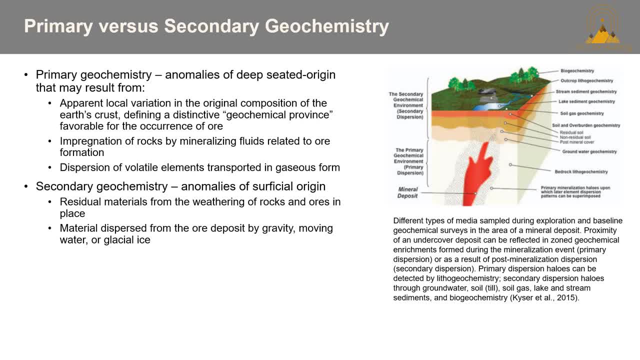 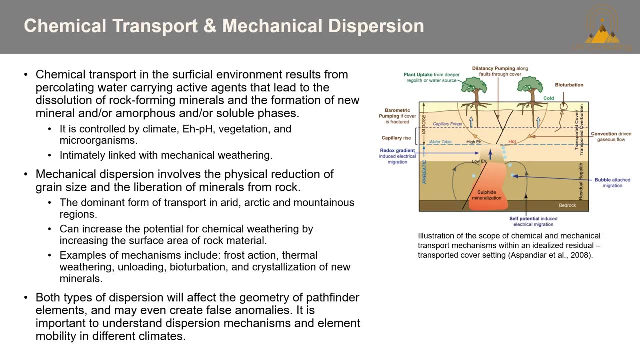 or as a result of post mineral dispersion: Primary halos detected mainly by lithogeochemistry and secondary halos through groundwaters, soils, tills, stream sediments, et cetera. Following this, the next important considerations are whether the area you're exploring 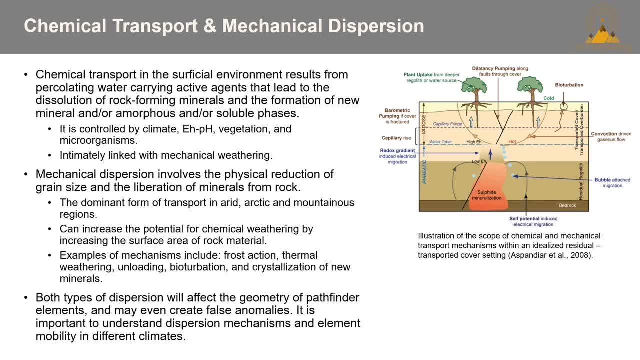 has been subjected to chemical transport or mechanical dispersion. Chemical transport in the superficial environment results from percolating water carrying activations that lead to the dissolution of rock forming minerals and the formation of new minerals or endomorphous or soluble phases controlled by climate. EHPH, vegetation microorganisms. 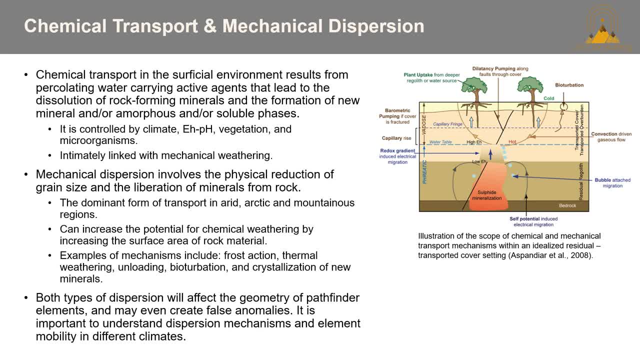 It's also intimately linked with mechanical weathering. Mechanical dispersion, on the other hand, involves the physical reduction of grain size and the liberation of minerals from rock. The dump form a transport in arctic and mountainous regions, and it can increase the potential for chemical weathering. 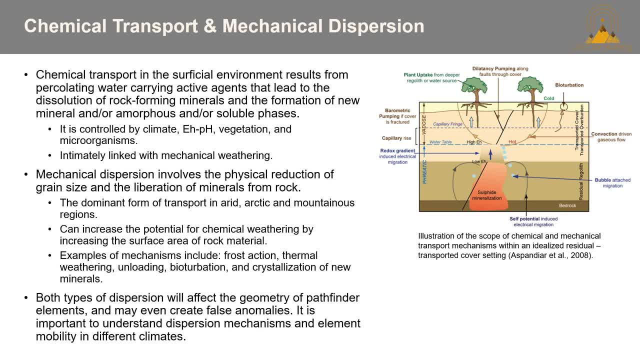 because it's going to be increasing the surface area of the rock material. And there's a bunch of examples: frost action, thermal weathering, unloading. Both types of dispersion will affect the geometry of pathfinder elements and may even create false anomalies. 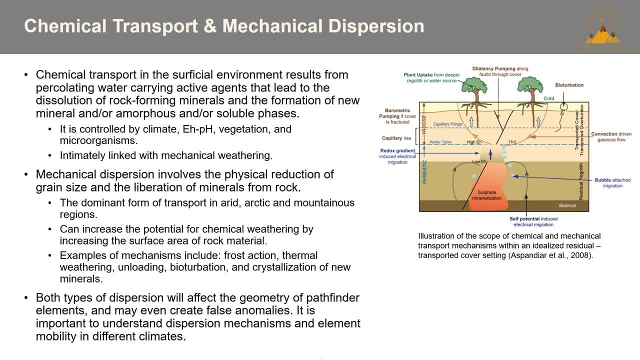 It's important to understand the dispersion mechanisms and element mobility in different climates. The illustration up right is an idealized version of a residual transported cover setting. There are a lot of considerations here We're going to take into account for something that potentially even may look a little bit simple. 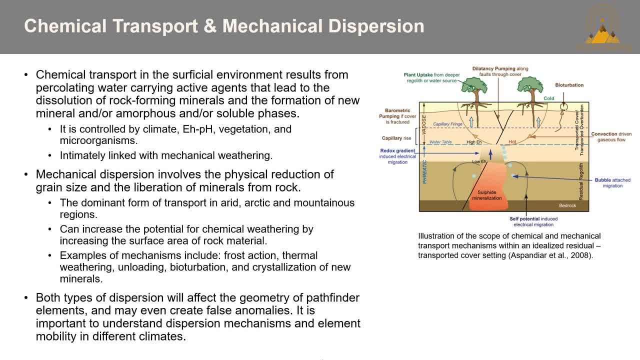 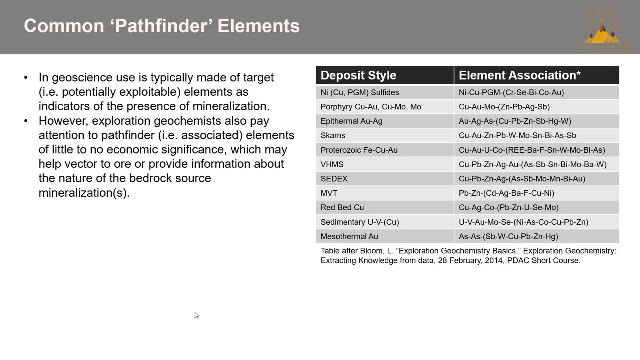 So it's really important that you know your climate, your geomorphology, the tectonics, even. It all adds the greater picture of what you're going to be seeing in your data. Commonly, large data sets are acquired, but perhaps only a few elements are used. 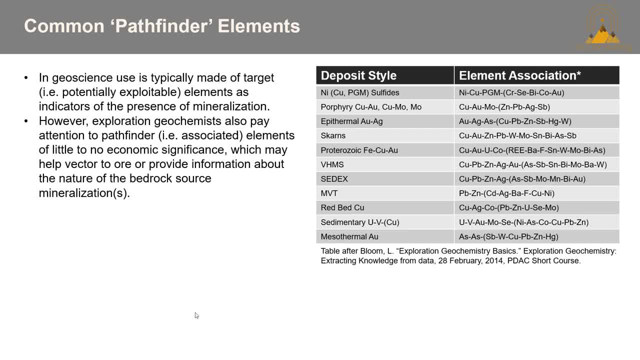 such as the ore elements and perhaps a few others. However, for many years of study, geochemists have found that. However, for many years of study, geochemists have found that there are elements that are associated with specific ore deposits that are useful to track. 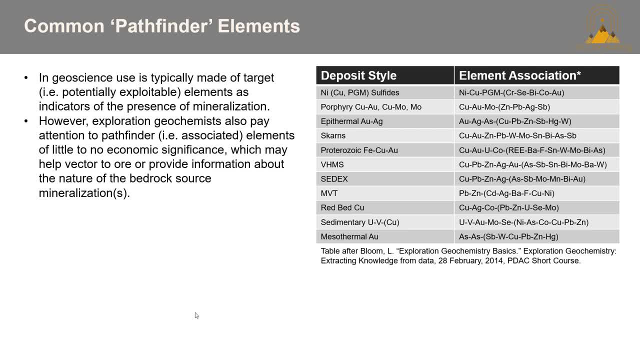 when looking for new systems, And these are called pathfinder elements. The table at the right is some good examples for different ore deposits, For example, epithermal gold silver. You could, in addition to seeing gold and silver, which hopefully you see would be arsenic. 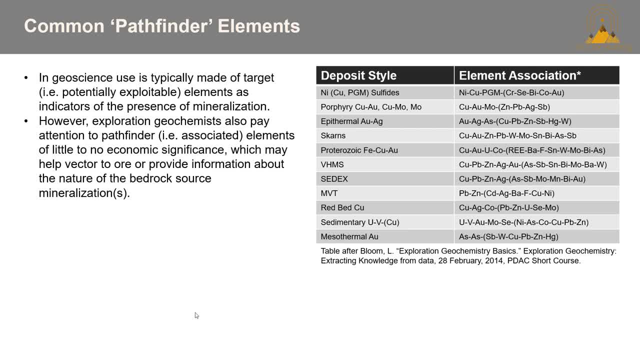 but also potentially, copper, lead zinc, antimony, mercury, tungsten. Each deposit is going to be different, but by looking at your data, you're going to be able to see that these are some good elements to have a start with looking at. 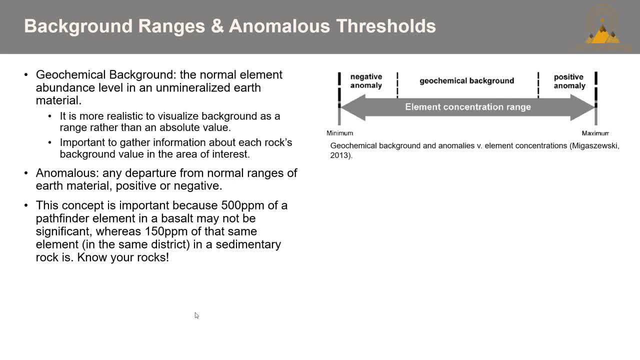 The last topic I want to touch on here is the concept of background ranges and anomalies. Geochemical background, that's the normal element abundance level in an unmineralized earth material. It's more realistic to visualize this as a range rather than an absolute value. 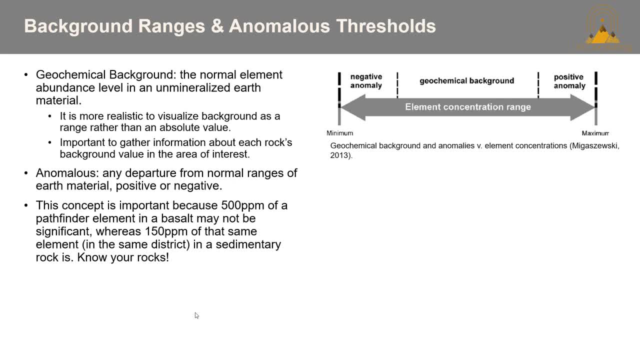 But I'm going to say that it's really important to gather information about- you know about each rock's background value in the area of interest that you're working in. An anomaly: is any departure from the normal ranges of the earth material positive or negative?